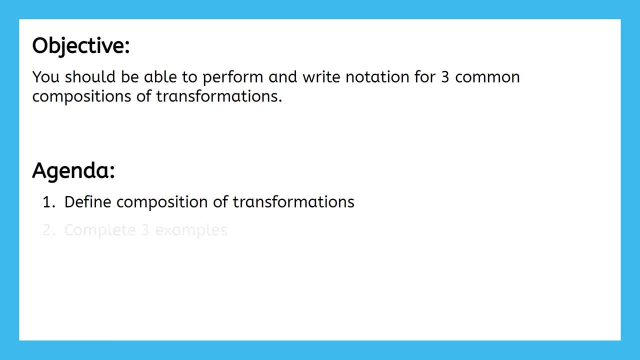 define composition of transformations, And then we'll complete three examples, one for each of the most common types learned about in geometry. So you're probably wondering what exactly is a composition of transformations? Well, this is what we call it when two transformations happen to the same figure, For example there: 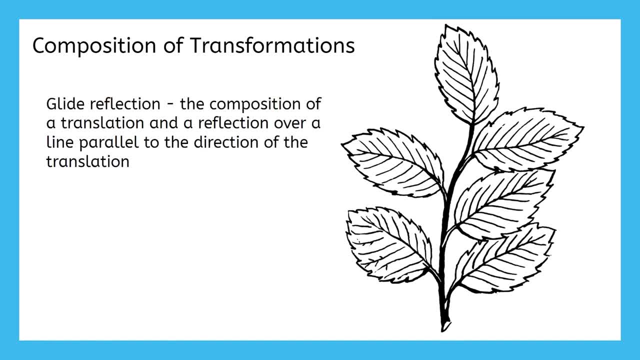 are many plants that have a glide reflection. A glide reflection is a translation and a reflection combined to get the image. It's like taking one of these leaves and shifting it up and then reflecting it to get the next leaf. Notice that we shifted vertically and then also reflected over a vertical line. These 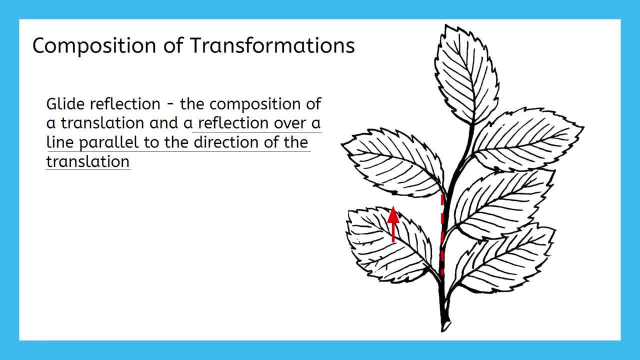 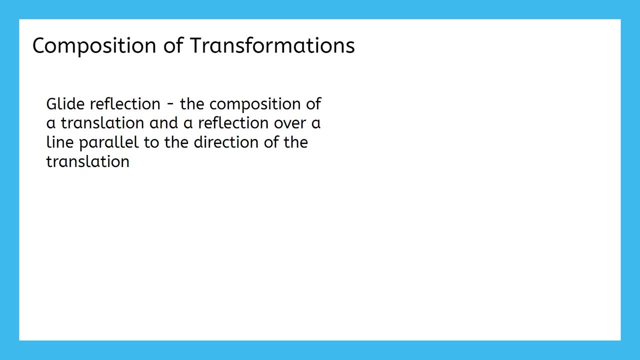 were parallel to each other, which is part of what makes this a glide reflection, since the direction of the translation is parallel to the line of reflection. A glide reflection is a composition of transformations, because it took more than one step to get to the image. 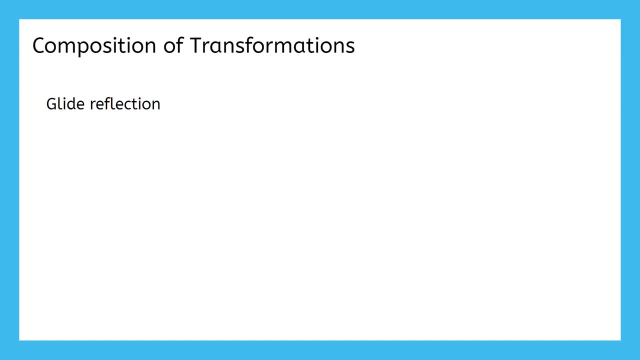 A glide reflection is one of the compositions we're going to do an example of today. In addition, we're going to look at reflections over parallel lines and reflections over intersecting lines. We're going to complete an example of each of these. so let's get started. 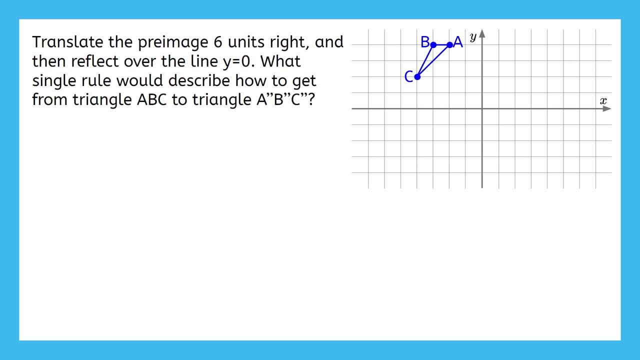 Our first of three examples is a glide reflection, like we just talked about. This says, to translate the preimage six units to the right and then reflect over the line y equals zero. What single rule would describe how to get from triangle ABC to triangle, A double prime? 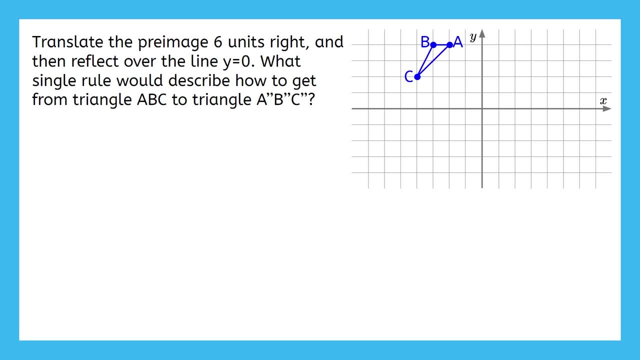 B double prime, C double prime. Yeah, this is the first time we're using double prime. This notation tells us that there's two transformations happening To get to our image. So there are two ways that you could approach this problem. Try to find the points on the preimage- first step and image- and write them down. 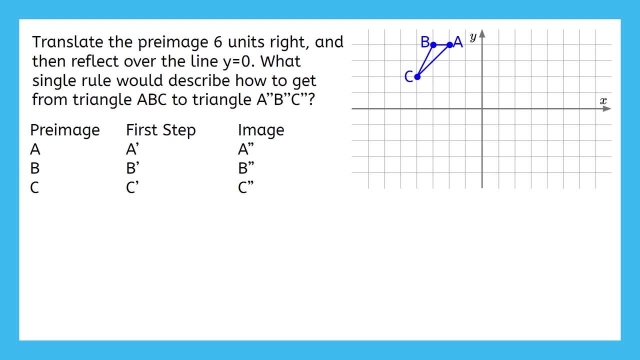 The first step will represent the points after the translation and the image will represent the points after the translation and reflection. You may choose to sketch on a coordinate plane to help you, or create and use the rules or coordinate notations for each step. 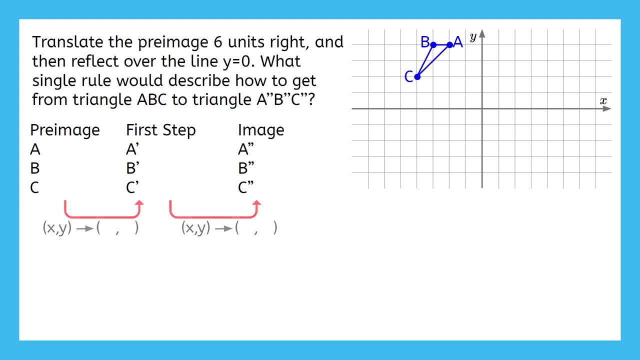 Let's take a look. It would be best to use both methods to make sure that you're confident in your answer. Pause the video now to try this, and then afterwards we'll talk about how to finish the rest of the problem. All right, it's time to check your work. 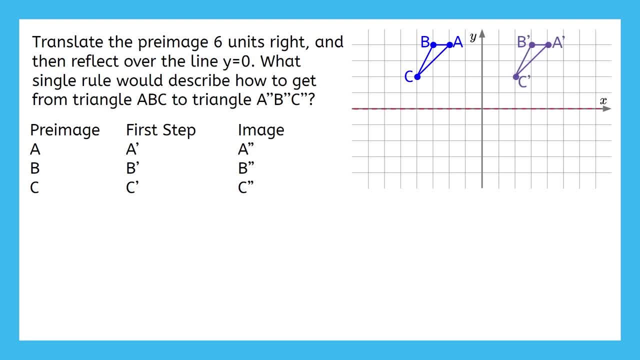 Here are the graphs of the first step when translating six units to the right, and the final image when reflecting over the x-axis. And here are the notations that help us to make each move. Let's take a look, Go ahead and pause the video here so you have time to check your work. 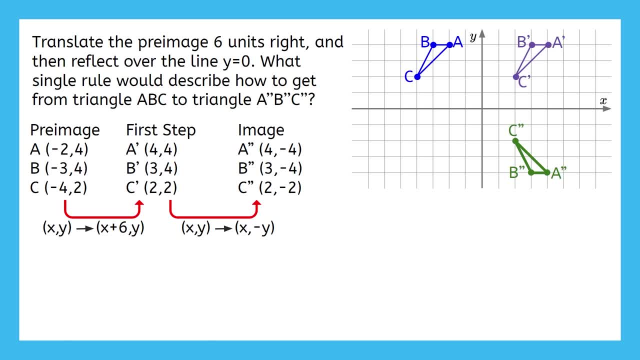 The directions are also asking what single rule or coordinate notation can take us directly from the preimage to the image. In other words, how can we bypass this step in the middle and only use one coordinate notation to describe both transformations? Remember finding patterns a bunch of times throughout this video. 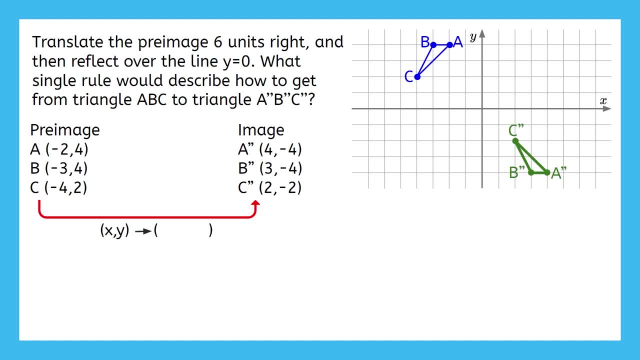 Let's take a look. Well, we have to do the same thing here. Take a moment here to figure out how to get from A to A'' and verify that this rule also works for the other points. The x values increased by 6, and the y values changed signs. 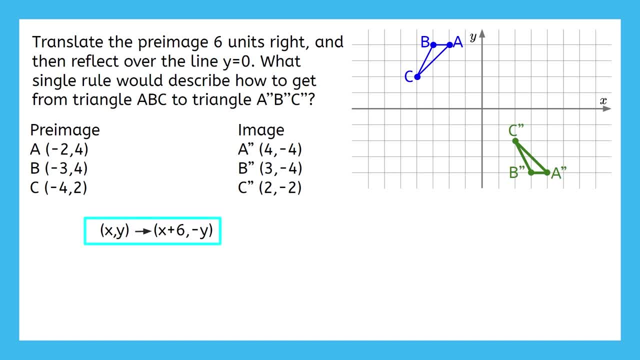 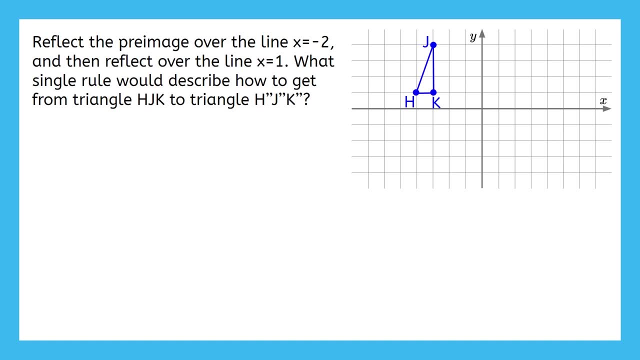 Here we have it, One single rule to take us through both transformations. Our second example involves reflections over parallel lines. This says: to reflect the preimage over the line x equals negative 2, and then reflect over the line x equals 1.. 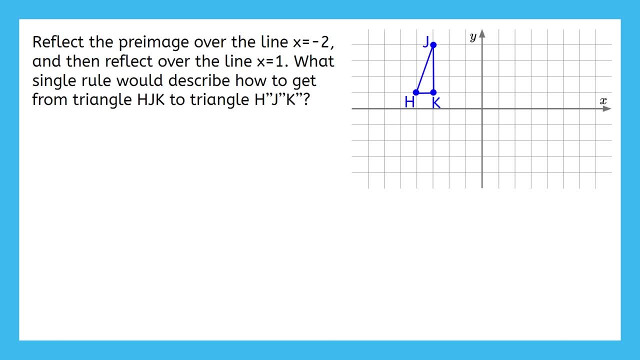 What single rule would describe how to get from triangle HJK to triangle H''J''K''? First, let's try to find the points on the preimage- First step and image- First step and image- And write them down. 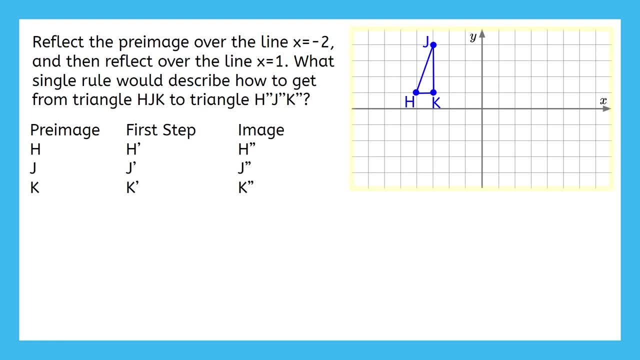 Sketching on a coordinate plane would be the easiest way to find the first step in image for this problem. Trying to figure out the notation for each step would be a bit tougher than making the sketches, but it is an option if you want to try it. 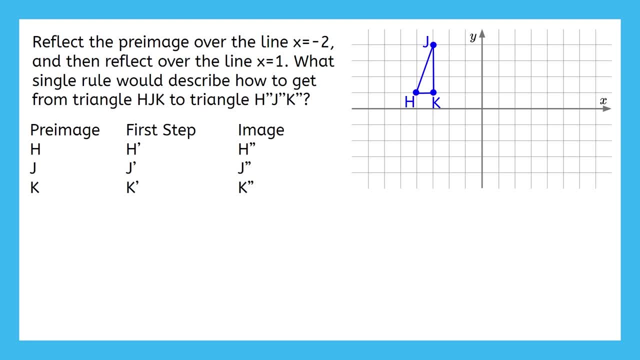 Pause the video now so you can work this out. Let's check your work. Here are the graphs of the first step: when reflecting over x equals negative, 2.. And the final image: When reflecting over x equals 1.. Since the directions are asking for a single rule, that can take us directly from the preimage. 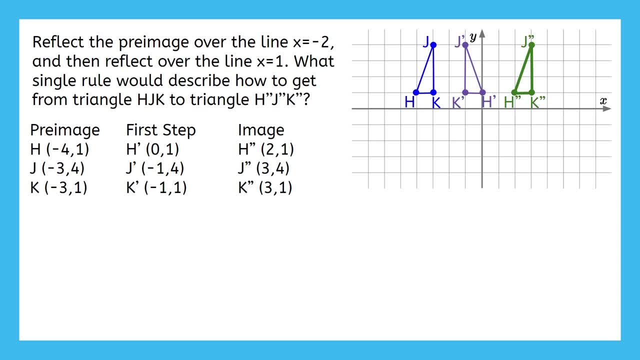 to the image. we want to be able to skip over the first step. Basically, let's bypass the step in the middle and only use one coordinate notation to describe both transformations. Take some time to figure out how to get from H to H'' and verify that this rule also works. 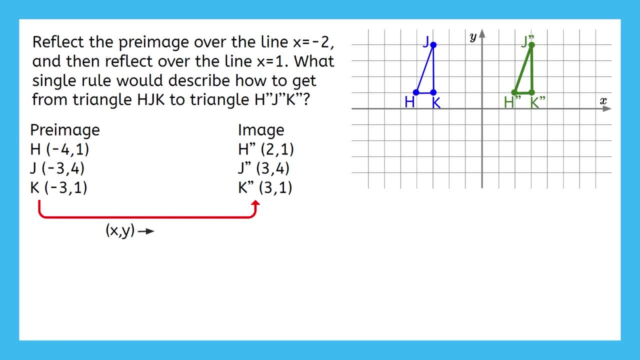 for the other points, Hopefully. you said that the x values increased by 6 and the y values stayed the same And actually the reason it became a horizontal translation by six units is because that's twice the distance between the two parallel lines of reflection. 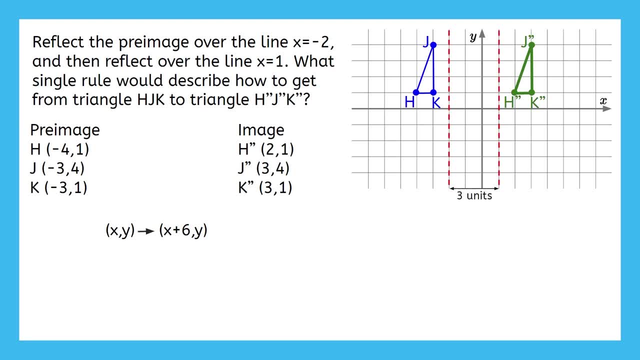 These lines are three units apart and multiplying that by two gives us 6., 3 units. over parallel lines the translation amount will be two times the distance between the parallel lines. Let's circle or box in our final answer so we can say: 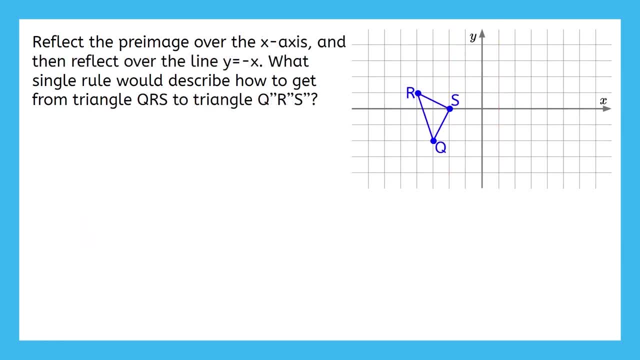 we've completed this problem. This is our final example for today, and this time we're supposed to reflect over the x-axis and then the line y equals negative x. Find the points on the pre-image, first step, and image using both methods, this time Sketch in a coordinate plane and create and use the. 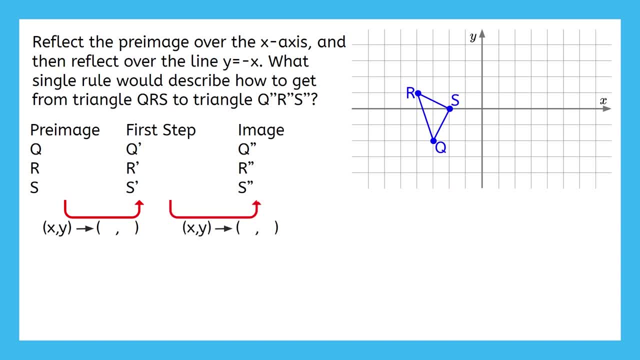 rules for each step. Using both methods this time will give you extra practice, ensure that you've checked your work and verify that you're comfortable with each. So pause the video now to try this on your own. Let's see how it went. 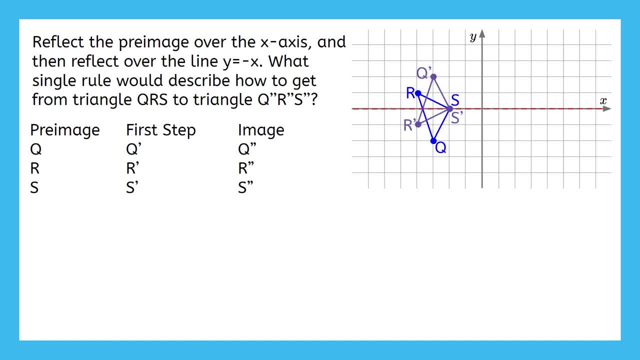 Here are the graphs of the first step: when reflecting over y equals 0,. and the final image, when reflecting over y equals negative x. And here are the notations that help us to make each move happen. Go ahead and check your work. The directions are asking what single rule can take us directly from the